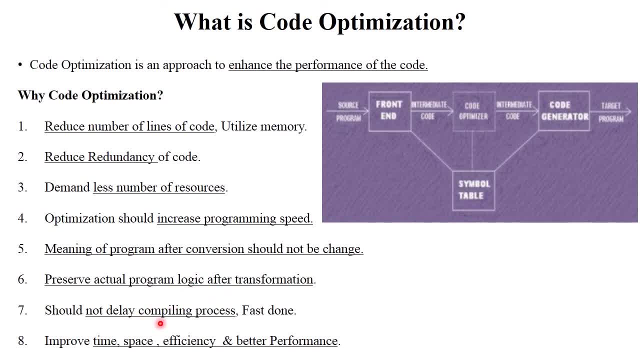 Okay, and it should not delay compiling process. It improve time, space efficiency and better performance of your program. So this is the reason that's why we use code optimization in your program. Okay, so code optimization is an approach to enhance the performance of your code. Okay, see here, this is a source program. Source program can be converted into the intermediate code. Okay, so what is intermediate code? How intermediate code is represented. 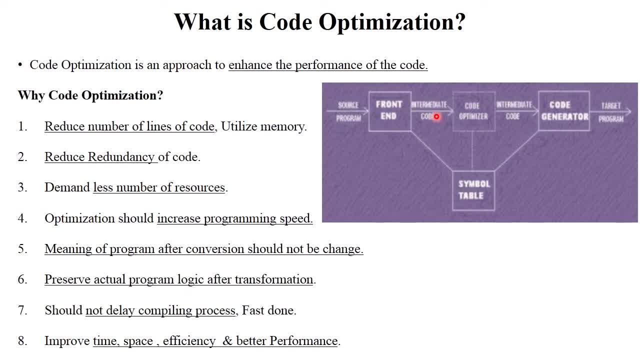 We already learnt in my previous video. Okay, so intermediate code is provide as an input to the code optimizer. Okay, so there is optimized the code through code optimizer And this optimized code provide as input to the code generator phase. Clear. So code optimization is second last phase of compiler- Clear, Okay. 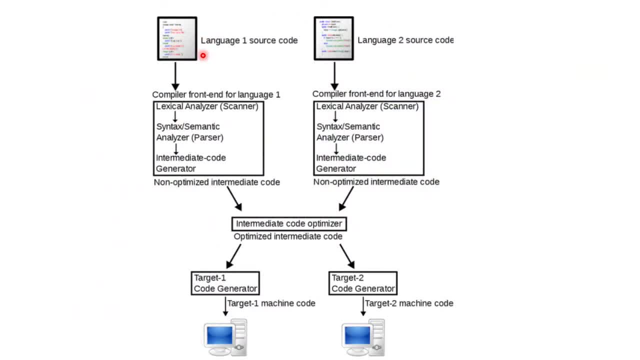 Say: this is a source code. Okay, source code after, when you compile your program: Lexical Analyzer: It analyze or scan all the tokens in your program. Then there is Syntax and Semantic Analyzer: It checks syntax and meaning of your program. And then there is: 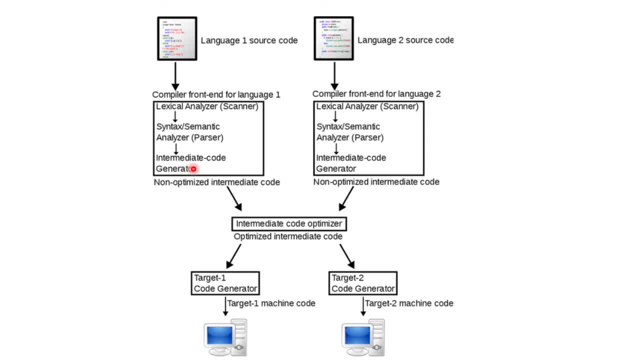 Intermediate Code Generator. Okay, So after intermediate code will be generated, it send to the Code Optimizer. It optimize your intermediate code and send this code to the Code Generator. Code Generator is the last phase of compiler And this Code Generator, or this, is machine. 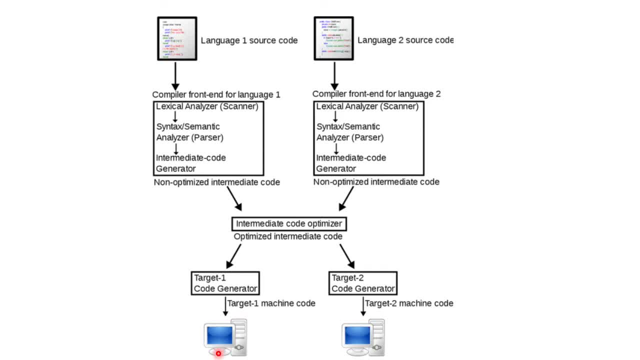 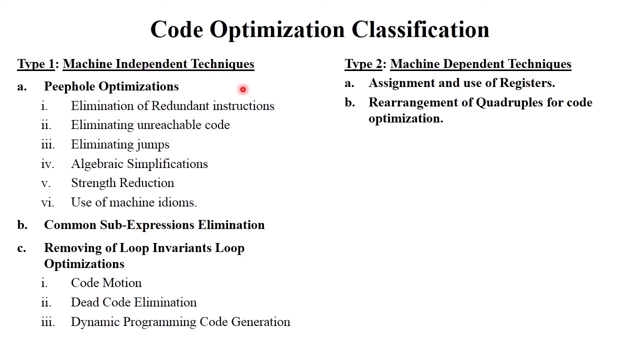 code can be executed on your system: Clear. So this is the complete structure of phases of compiler. In this way your program is compiled, Clear, Okay, Optimization Classification. There are two types: Machine Independent Techniques and Machine Dependent Techniques. Machine Independent Techniques have Peephole. Optimization Common: 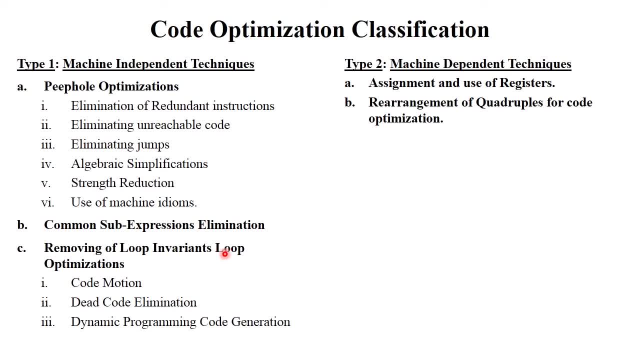 Sub-Expression Elimination, Removing of Loop Invariants: Okay, And Machine Dependent Techniques have again two types: Assignment and Use of Registers, Realization of Registers and Arrangement of Quadruples for Code Optimization, Clear. So let's see, one by one, how exactly. 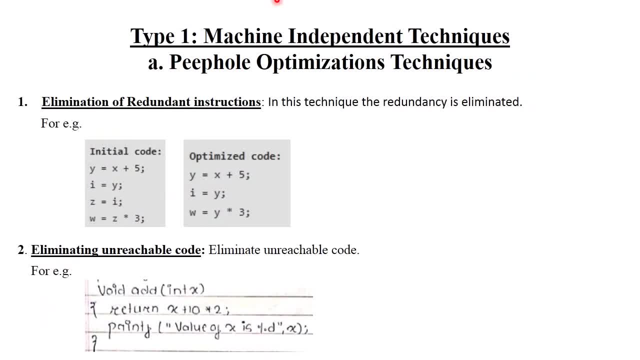 Code Optimization work Here. first is Peephole Optimization Technique. Okay, So in Peephole Optimization Technique the first task is to eliminate redundant instruction or duplicate instruction in your code. See here: this is initial code. X plus Y can be stored in Y. 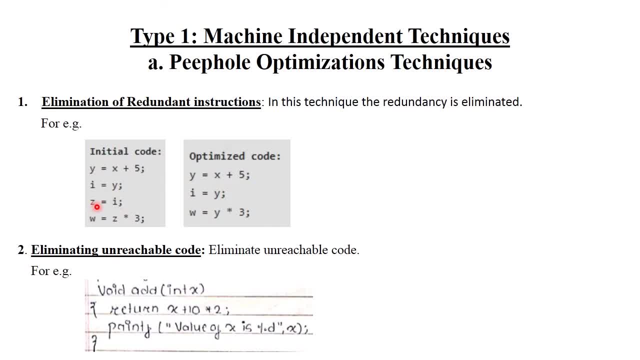 Y can be stored into I. I value can be stored into Z. Okay, And last, Z into 3 can be stored into W. See here, if you store Y value into I, then this code is not valid, Okay, Because? 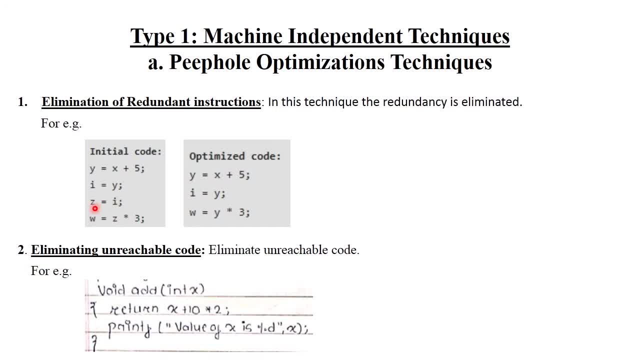 this is duplicate code. Okay, So you need to eliminate this code because you can store directly Y and I value into this Z. Okay, So this is optimized code. You just write Y value can be stored into I and you write Y or I value into 3 and it can be stored into. 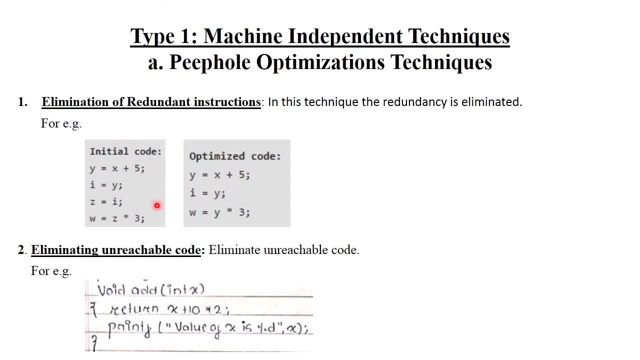 W Clear. So eliminate redundant instruction. Clear The next one to eliminating unreachable code. Okay, See, here the given function is void. add int X. Okay, The first statement is return. Return X plus 10 into 2 and after. 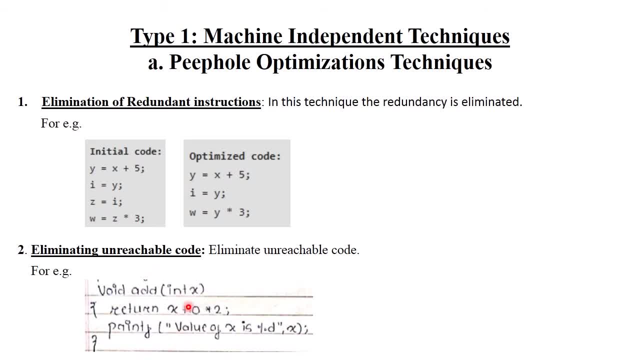 that print statement is executed. Okay, But in this function after return statement, the cursor doesn't go on this next statement. Okay, So you eliminate this unreachable code. Okay, In first statement is return their value into this function. Okay, So eliminate this. 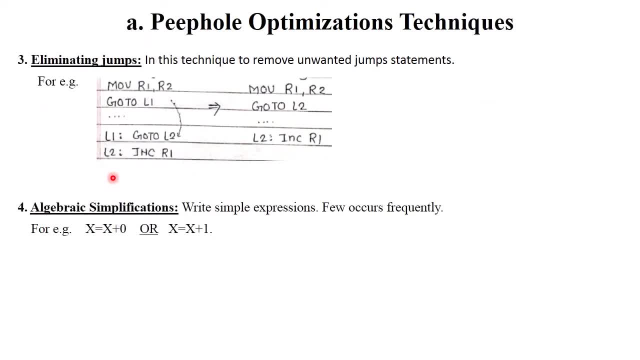 unreachable code. Clear, Okay. Next one is eliminating jumps here Okay, To remove unwanted jumps from the your program. See here: this is initial code: Move R1, comma R2, then go to L1.. Go to is used for jumping statement, So jump onto L1.. L1 is go to L2.. Now jump. 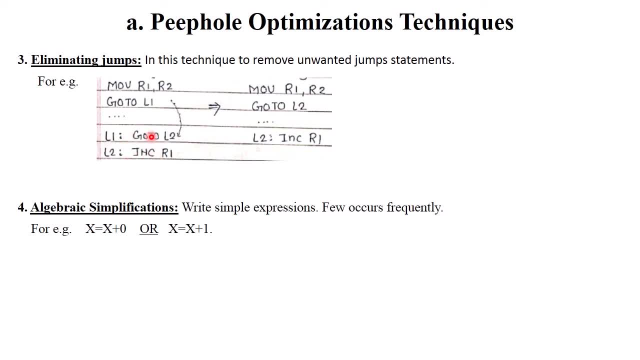 onto L2 statement Clear. But there is no necessary for this statement. So optimize code in this way: Move R1 comma R2.. Go to L2.. Okay, You can directly jump on L2 statement, Increment R1.. Okay, So you remove. 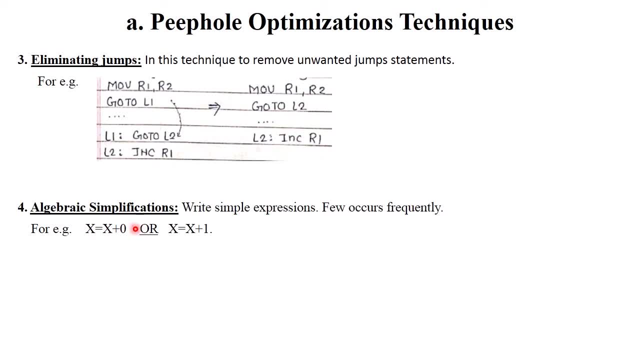 this unwanted jump statement Clear. So next one is algebraic simplification. Algebraic simplification means simple expression which occurs frequently in your program. Write X equal to X plus 0, X equal to X plus 1.. Okay, So you should use algebraic simplification. 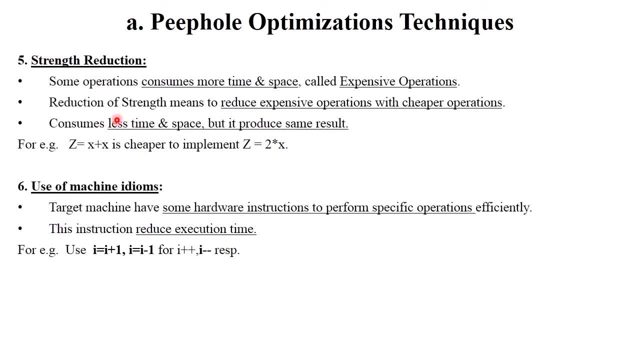 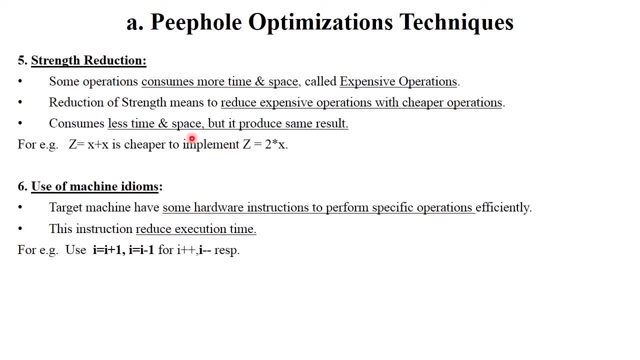 Okay, So strength reduction means to reduce expenses. So strength reduction means to gegeben information product and to reduce expenses by 사용 arrangement flows. So this is tahun Ettan efficiency, Stanford University. Now you can see here it is now more aoE. So if I willifting again, So this is what. 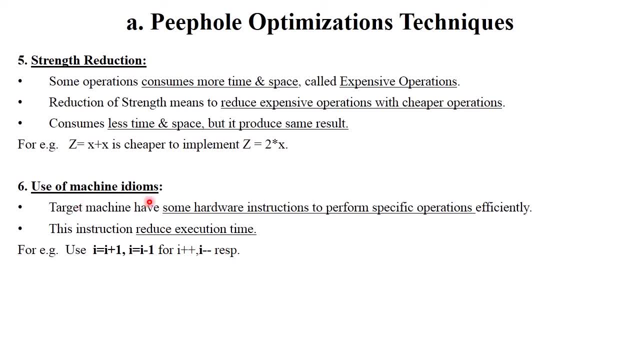 it will be like is that you can see the difference. I can have всего more operations between Clear. Next one is use of machine items. Okay, Target machine has some hardware instruction to perform specific operations efficiently. Okay, It reduces execution time. Okay, So you should use. 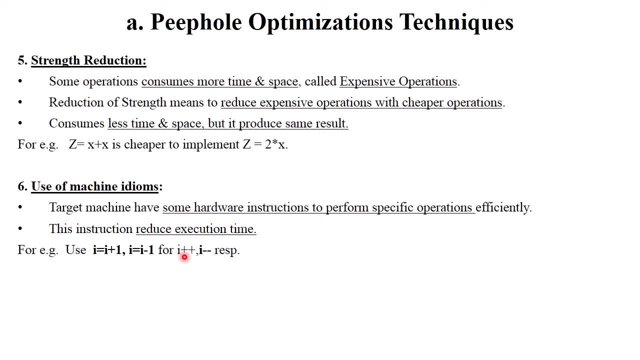 i equal to i plus 1, then i plus plus. Okay, Then i minus minus. you should use i equal to i minus 1.. Okay, This requires less time and less space. Okay, So this is called peephole optimization. 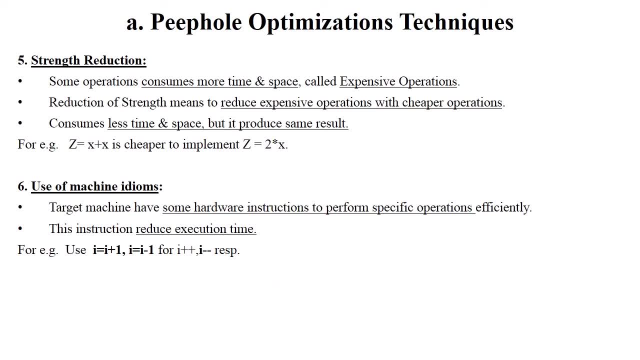 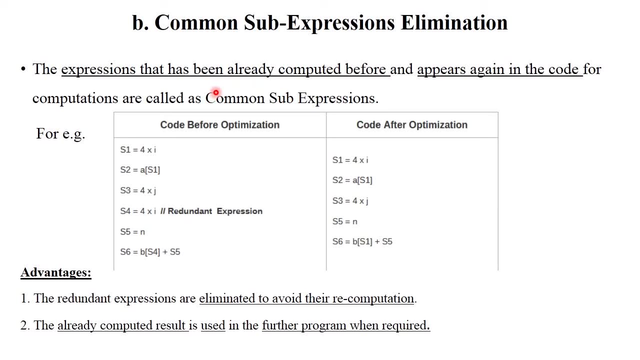 technique. You should use this optimization technique while doing program. Clear: Okay. Common sub-expression: elimination: Okay, The expression that has been already computed before and appears again in the code. This is called common sub-expression. Okay, See here. This is: 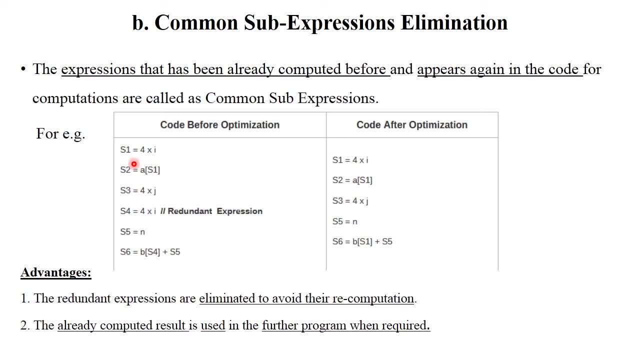 code before optimization: 4 into i. This value can be stored into s1.. Array of s1 can be stored into s2.. Then 4 into j. This value can be stored into s3.. Okay, Again, there is a common sub-expression: elimination. Okay, So you should use this optimization technique. 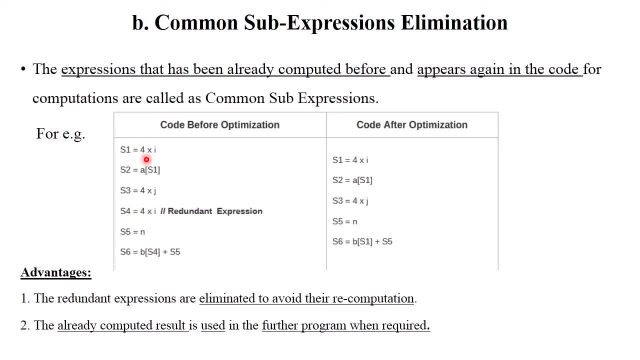 4 into i. That value can be stored into s4.. So this is called redundant expression or duplicate expression. Okay, 4 into i value is computed before in the program. Okay, So there is no any need to again. you can write this expression here. Okay, Then you should eliminate this. 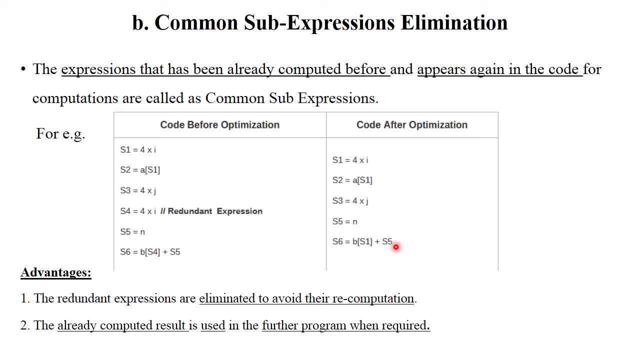 expression and this is your optimized code here: Clear. So advantages of common sub-expression is eliminated, recomputation time: Okay, And already computed result is used in the further program when required. Clear. So this is all about common sub-expression elimination. Next is removing of loop invariants and loop optimization. So 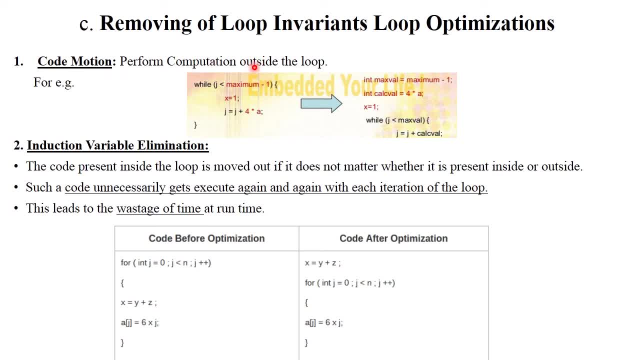 first task is code motion. Code motion is perform computation outside the loop. Okay, See here In this example, while j less than equal to maximum minus 1.. Okay, So maximum minus 1 is computation. It requires computation many times when this condition is executed. 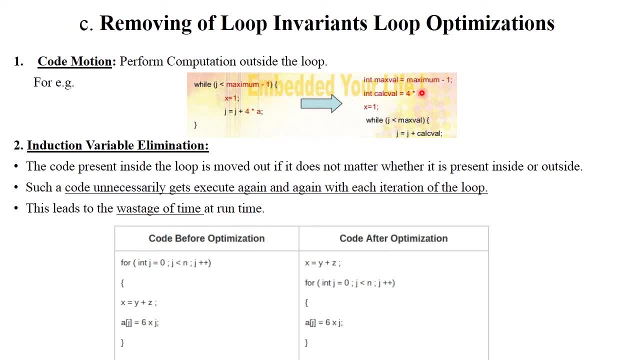 So optimize code in this way. You just calculate maximum minus 1 value and stored into one variable, That is max value. Okay, And you should use this variable into this condition. Clear. So computation time is much less here in optimized code. Clear, So this is called. 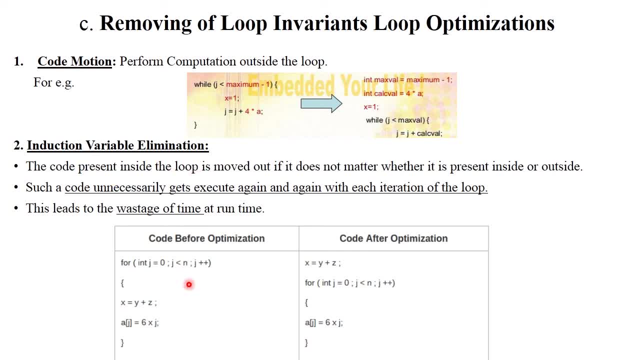 code motion, Then induction variable elimination, See here. Induction variable means code unnecessary gate, execute again and again with each iterations of loop. It leads the western direction. So this is called code motion. So computation time is much less here in optimized code. Okay, See here. 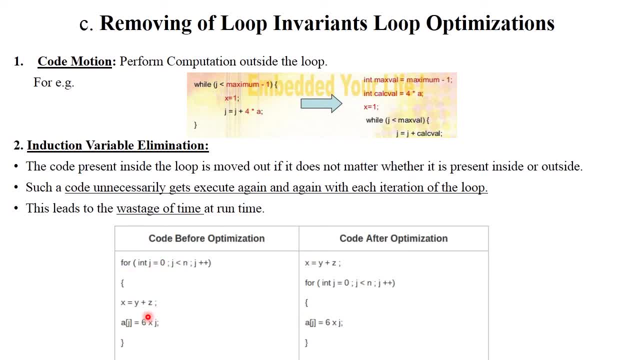 Code before optimization. This is for loop. When this for loop is executed, these two statements are executed: x equal to y plus z and 6 into j. Okay, But x equal to y plus j. it requires more computation. Okay Means as much as time this condition is executed, this statement is executed. 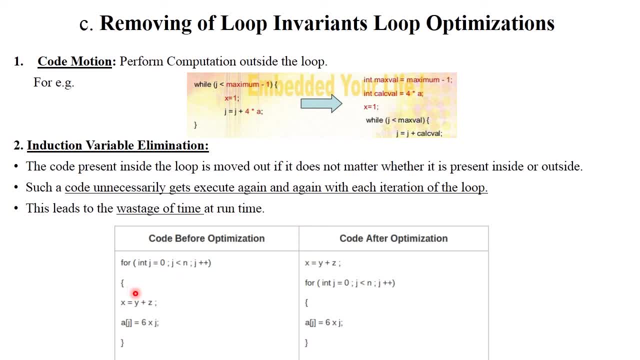 It requires more time. Okay. So after code optimization, this computation statement is executed before the loop. Okay Means it can be executed only after the loop is executed. So only one time Clear. So this is called induction variable elimination. Now next one is dead code. 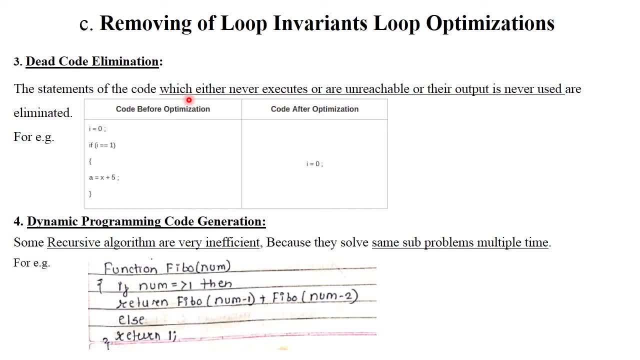 elimination. Dead code means the code which either never execute or are unreachable, or their output is never used. This code is eliminated, Okay. See here This is code before optimization: i equal to 0. Okay, But next one is: if i equal to 1,, then this code is executed: Okay, This is dead. 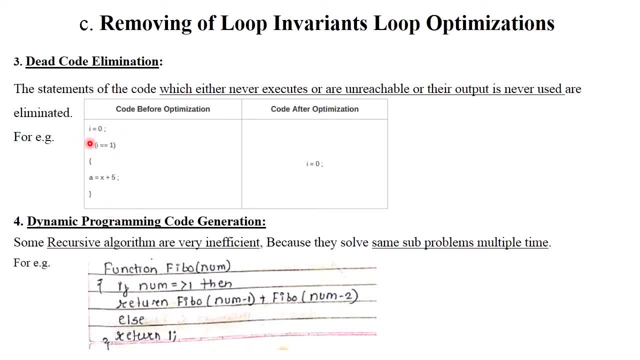 code. Okay, This is unreachable code, So eliminate this dead code Here. Okay, Now, after code optimization, the code is: i equal to 0., Clear, Okay. Next, dynamic programming: code generation. Dynamic programming simply means recursive algorithm. Okay, Which is. 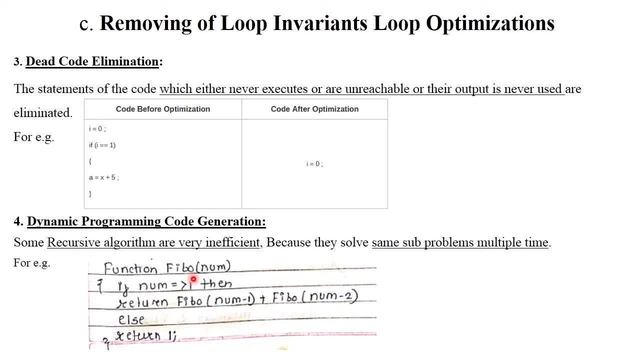 inefficient. See here: This is Vibonacci series. Okay, And recursively call this Vibonacci series again and again here. Okay, So remove this dynamic programming code generation. Okay, It solves same sub-problems multiple times, Clear, Okay. 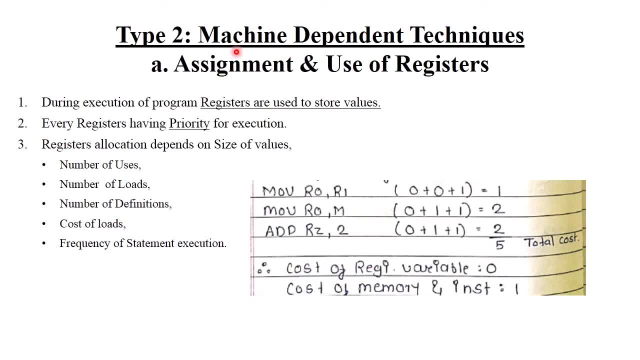 This is machine dependent technique. This is the second type of code optimization. Okay, The first one task is assignment and use of registers. You should use registers during execution of program. Registers are used to store the value. Okay, Every register is having priority for. 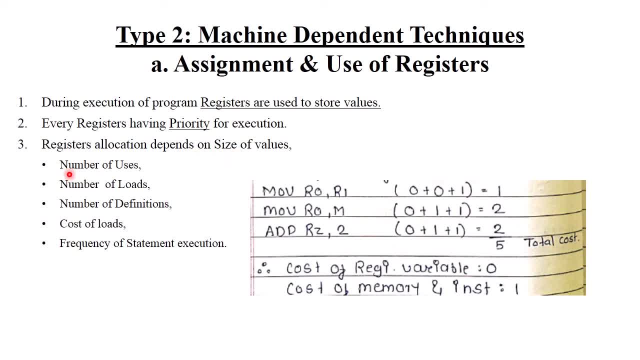 execution and register allocation depend on size of values, That is, number of users, number of loads, number of definitions, cost of loads and frequency of statement execution. Okay, See in here the cost of registers is 0 and cost of memory and instruction is 1.. Okay, Now see here: Move. 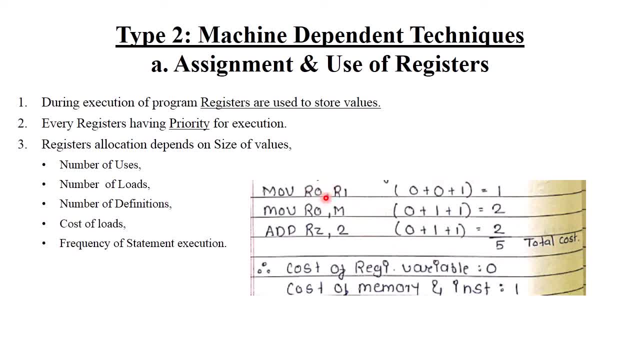 r0, r1.. This two is registers were stored. any value. Okay, So cost of register is 0 and 0.. And cost of instruction is 1.. Okay, So total cost is 1. Same here and same here in this also statement. So. 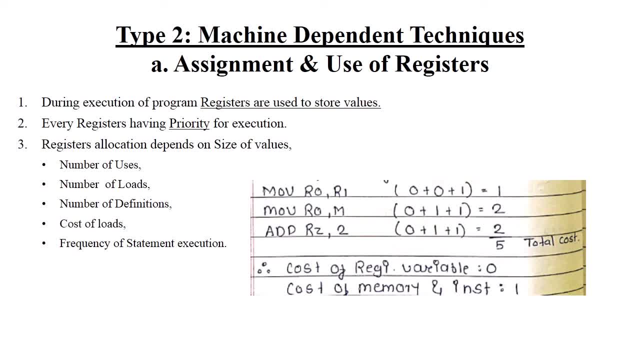 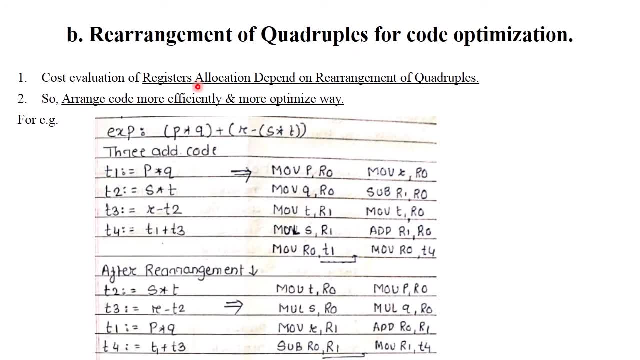 total cost become 5.. This is called assignment and use of registers. Clear. Okay For this. rearrangement of quadruples for code optimization. Okay. So cost evaluation of register allocation depend on rearrangement of quadruples. So arrange code more efficiently and more optimized way. Okay, You should analyze this example From this. 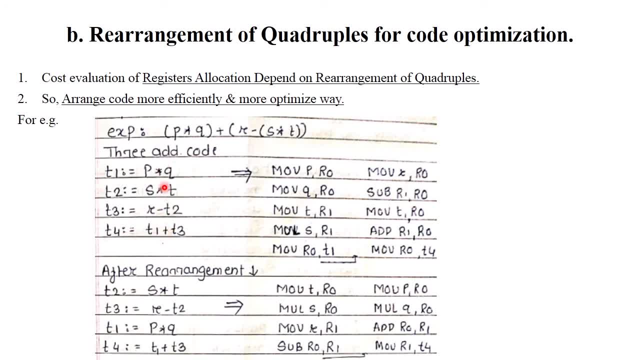 equation: this three address code is generated. And from this three address code, these instructions are generated. Okay. And after rearrangement this three address code, again these instructions are generated. Okay, You should analyze these examples. Okay, This is difference between machine. 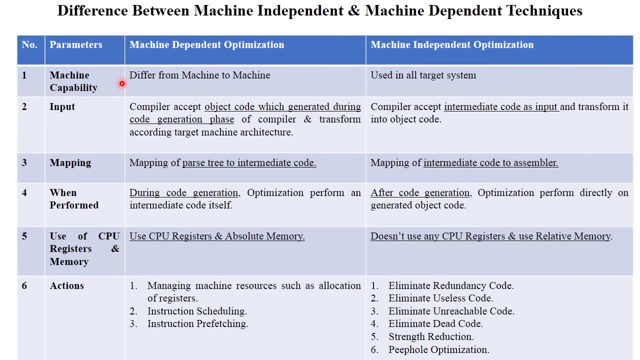 dependent optimization technique. Machine dependent optimization have machine capability differ from machine to machine. And machine independent technique: is used in all target system: Okay. Machine dependent optimization in accept the input as object code which generated during code generation phase: Okay. And machine independent technique has input is intermediate code: Okay, In machine. 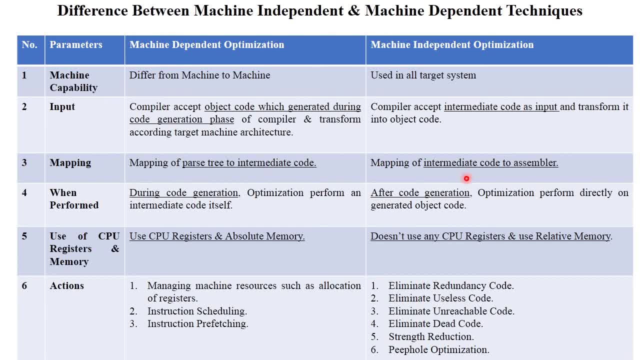 dependent, there is mapping of pass-through to intermediate code And in machine independent technique there is a mapping of intermediate code to the assembler. Okay, So machine dependent technique is performed during the code generation phase- Okay, And machine independent technique can be performed after the code generation phase- Okay. Machine dependent technique is: 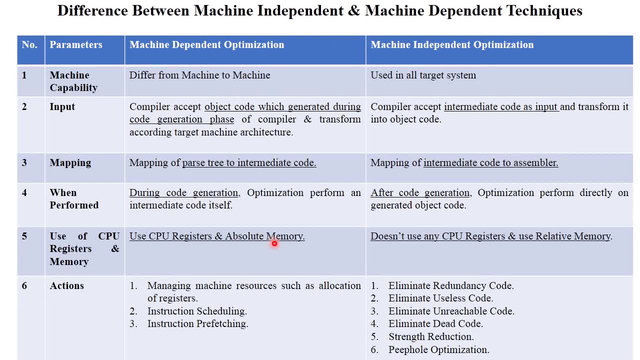 used CPU registers and absolute memory location. That is permanent memory location. Okay, But machine independent technique doesn't use any CPU register, It use relative memory reference. Clear. In machine dependent optimization these actions are performed Like managing machine resources, instruction scheduling, instruction prefetching, etc. But in machine